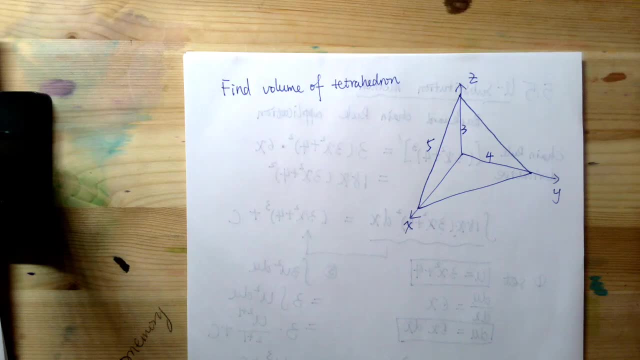 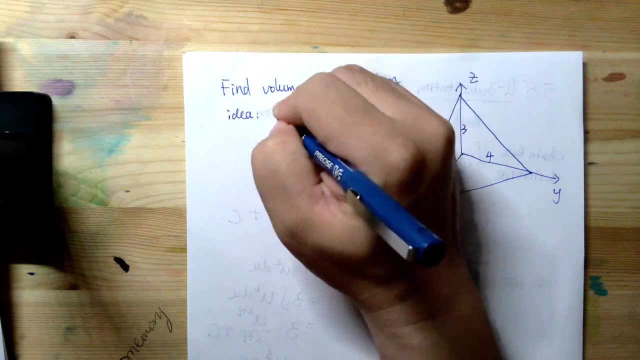 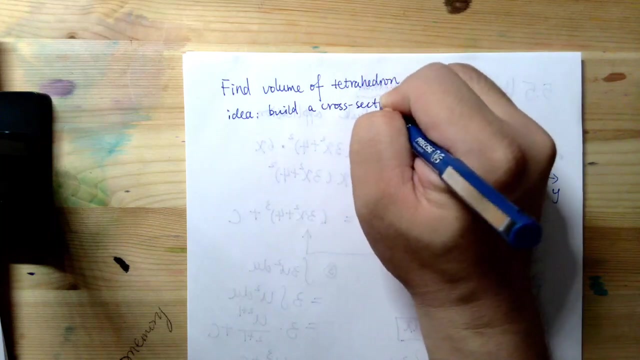 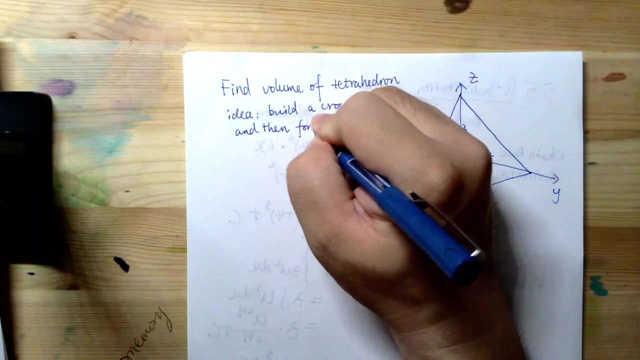 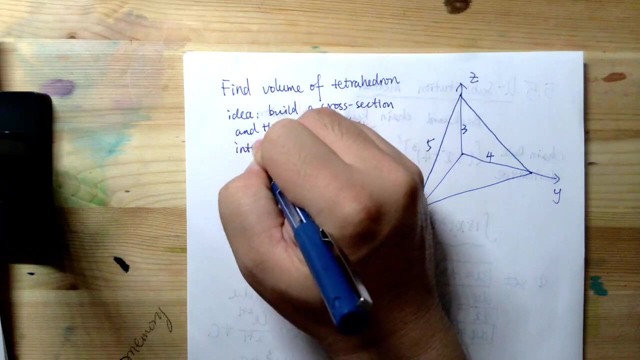 Okay, so the basic idea is to construct a cross-section and then set up the integral. Okay, so the idea is to build a cross-section and then formulate the integral. Okay, so that's how do we, how do we do So? 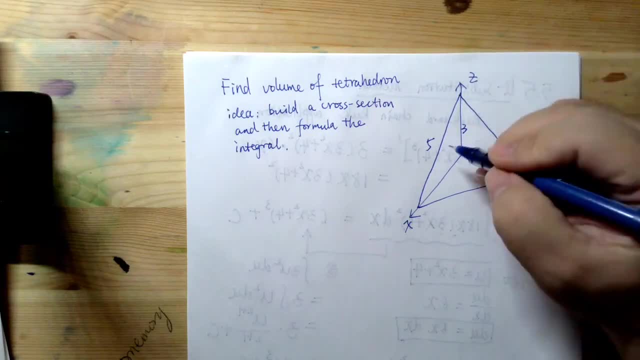 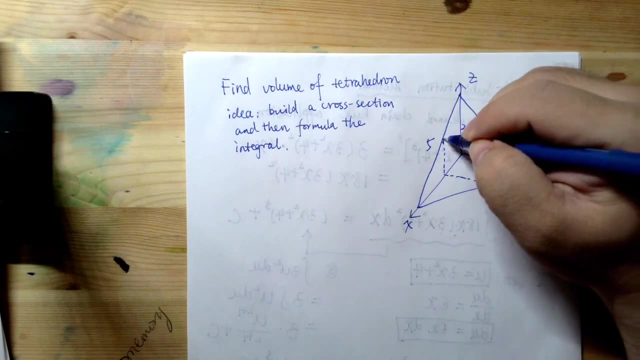 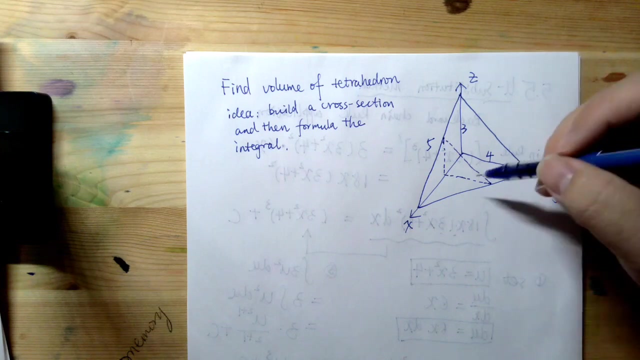 So, for example, how do we you know, if you construct a cross-section and such that it is perpendicular to the x-axis, So this is a cross-section and, as you can see that this is also a right, So this is a cross-section and, as you can see that this is also a right triangle. 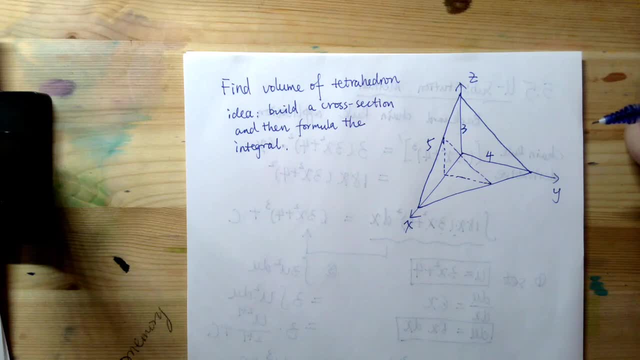 Okay. so so, based on the piece of Garvin's theorem, we can do some calculation. This is 3, this is 4, so this is hypotenuse for here, This is 5. also Okay, and also, you see, this is 5, this is 3.. 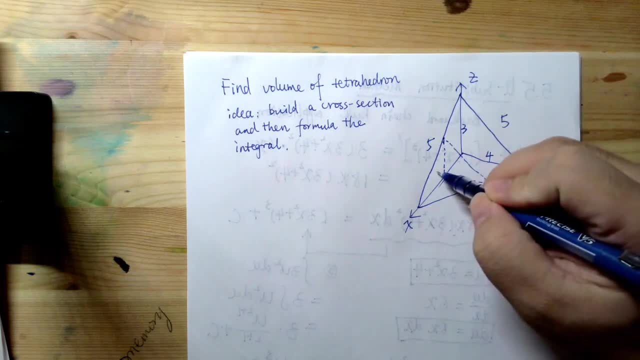 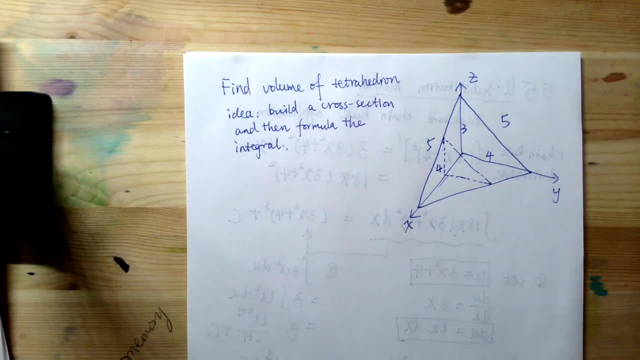 It turns out that the last for this is also 4.. Okay, also 4, maybe we put the 4 here. Okay, this Now, if we want to denote the length for this part as x, Okay, and why we do that? because you know, by constructing a cross-section perpendicular to x. 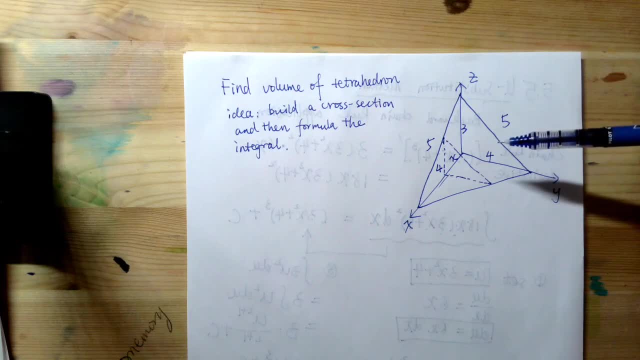 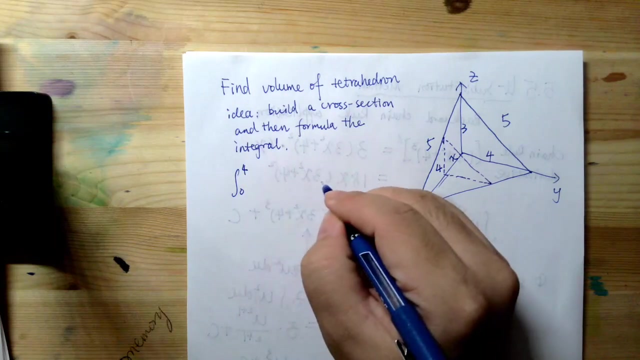 then I know that my integral is going to, along with x, and also I already calculated, the length is 4.. So the integral is 4. Okay, Okay, Okay, Okay. So I'll have it going to be something like you know, from 0 to 4, something dx. 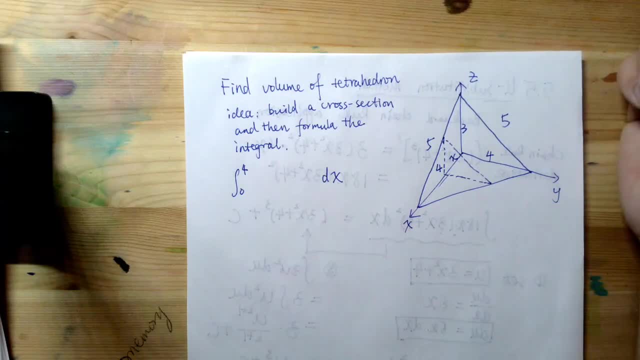 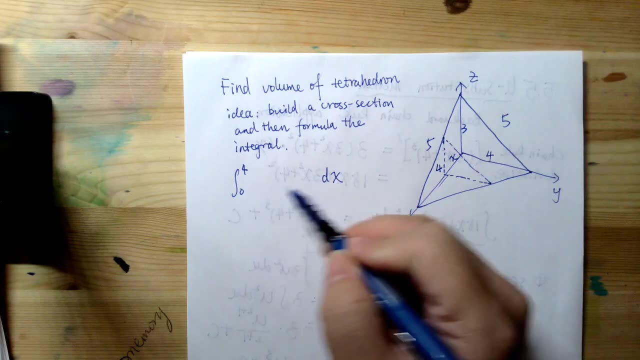 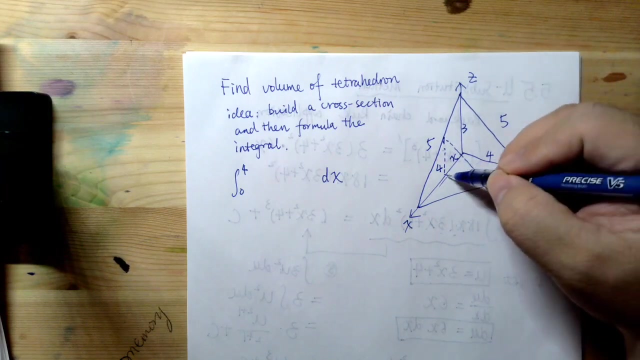 Okay, so that's going to be the pre-setup. Okay, but how do we find about the area of this cross-section? That's going to be the main task. Okay, So, as we know that if we set this part as x and then correspondingly the length for this part, 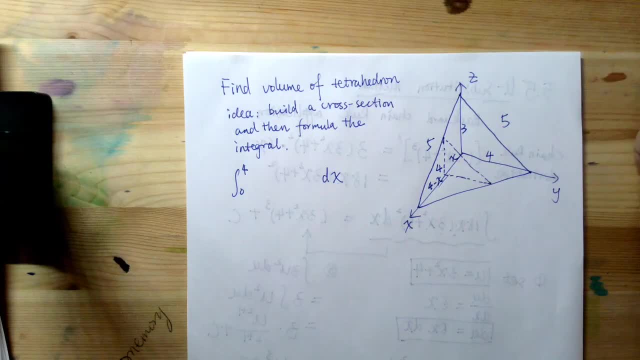 which is 4 minus x. okay, because total length is 4.. Now, if we denote, this is the height- okay- of this triangle for the cross-section, and we want to denote height in terms of x, Okay, And similarly, if I denote the length for this part, maybe we denote it as l. 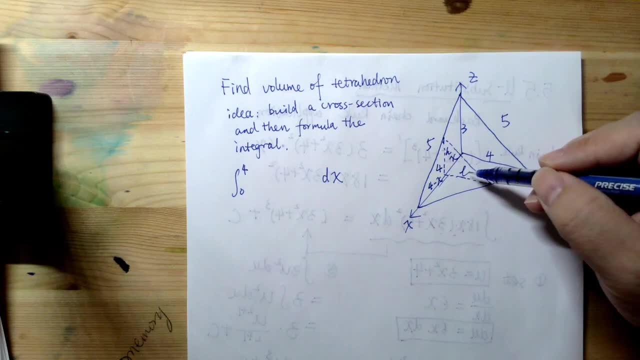 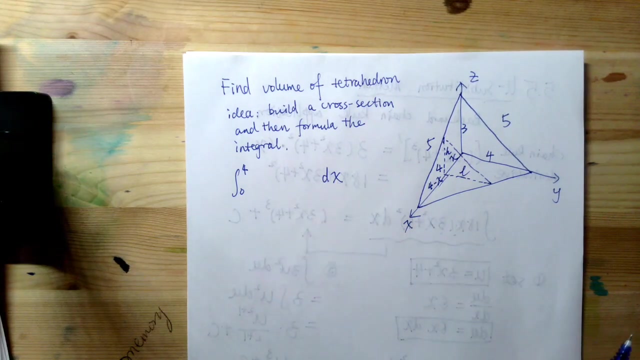 And then we also want to find an expression for l in terms of x, such that I can construct the area of this cross-section in terms of x, and then I can put into this integral here. Okay, So that's going to be the volume. 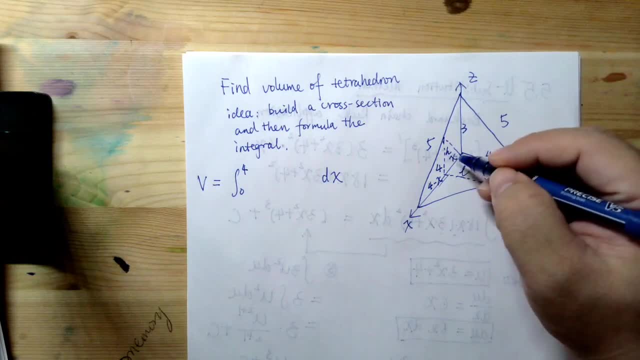 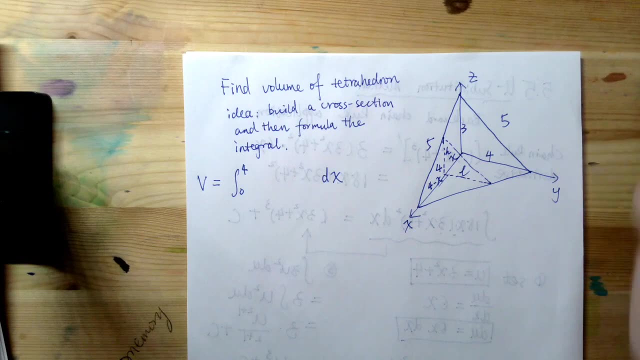 Okay, The volume. So how do I find h in terms of x and l in terms of x? Well, this is what we can do. If we only look at the x-z plan, okay, and you know, this is the x-z plan and we actually 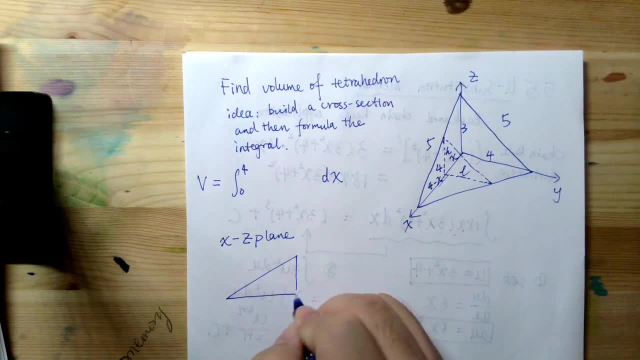 can draw that you know. so this is 3,, this is 5, and then you know this is 4,, and then you know this is h, right, This is x, This is 4 minus x, and, as you can see that this small triangle is similar to the larger, 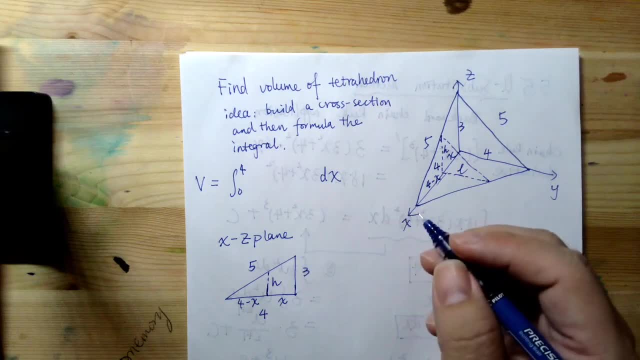 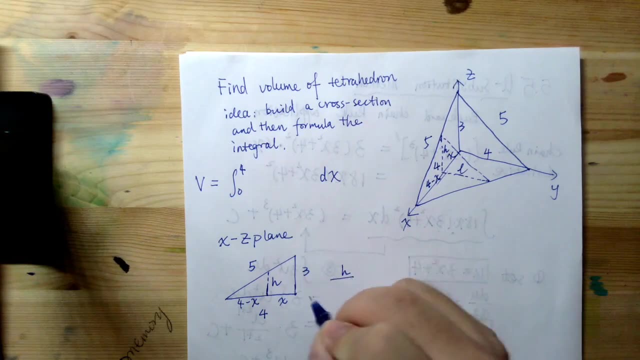 triangle. Okay, And then the ratio of the sides actually is going to be the same, meaning h over 4 minus x. you know, the ratio of this over this are going to be the same, Okay. Okay. So we can find h is 3 over 4 times 4 minus x. 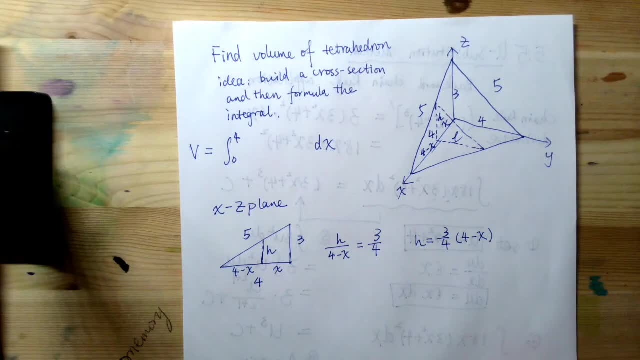 Okay, So that's what we can do here. And then, similarly, to find l in terms of x, we look at the x-y plan. Okay, And we can draw the x-y plan, Okay. And then, similarly, to find l in terms of x, we look at the x-y plan. 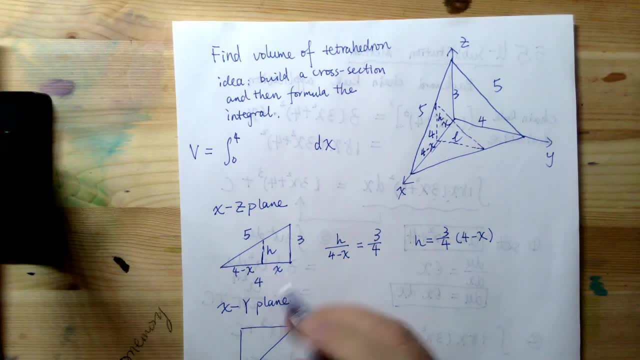 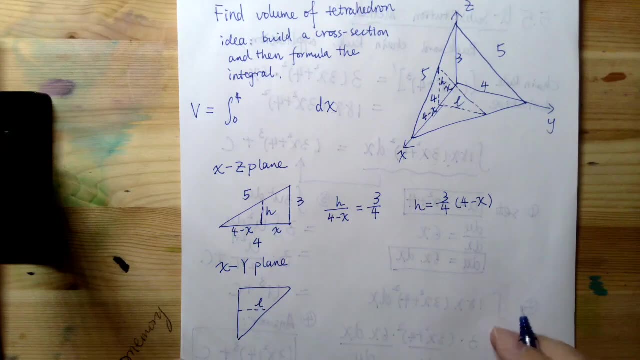 And then we can draw the graph and you can see: this is l, right? So suppose this is x. This is 4 minus x, right? So the over last for this is 4.. This is also 4.. 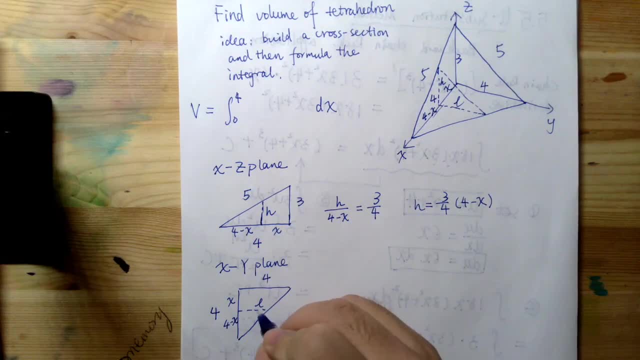 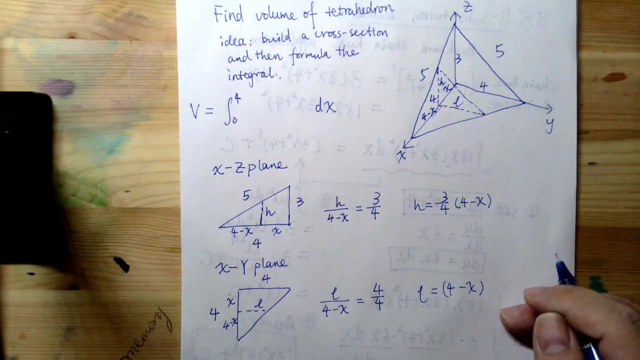 So this one is easy, right, Because you can say similar things. small triangle is similar to this larger triangle, so L over 4 minus X equals 4 over 4. turns out L equals 4 minus X. okay, and with this, so you can see that the 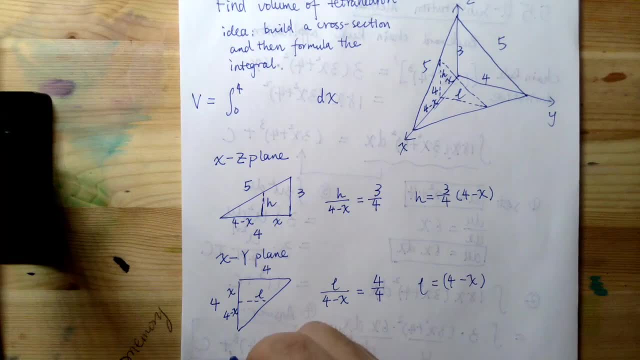 area for my cross-section is: area is 1 over 2 right high times L, which is 1 over 2, times 3 over 4, 4 minus X and then times 4 minus X. okay, turns out it's a 3 over 8, 4 minus X. 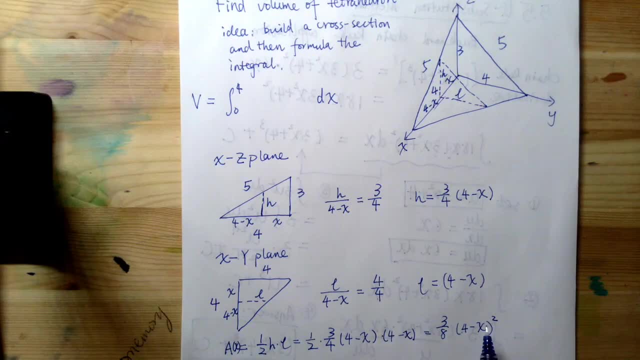 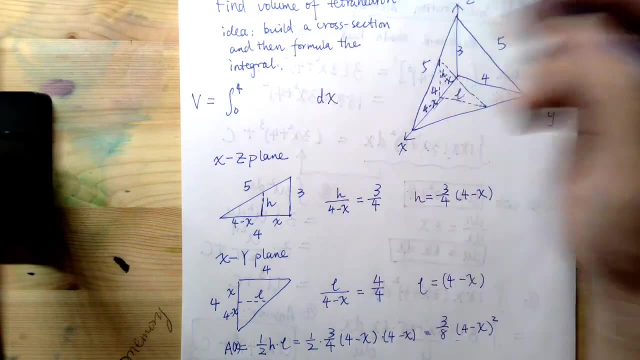 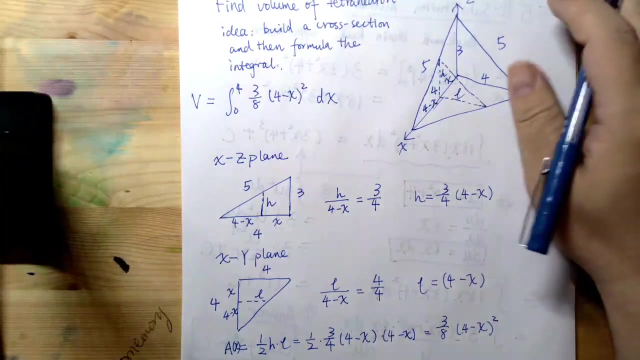 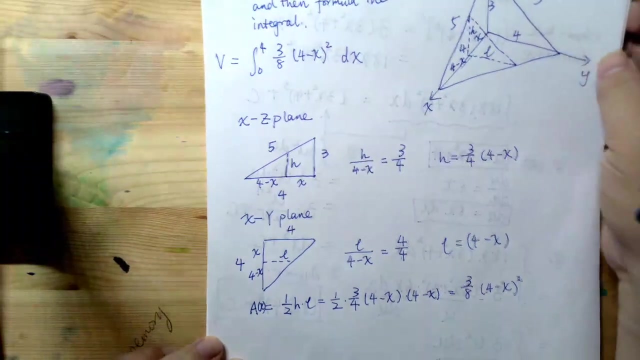 square. so this is the area for the cross-section. that's exactly what we're going to put back to this interval, which is 3 over 8, 4 minus X square. okay, so the following part is just to evaluate this integral, which is: V equals from 0 to 4. 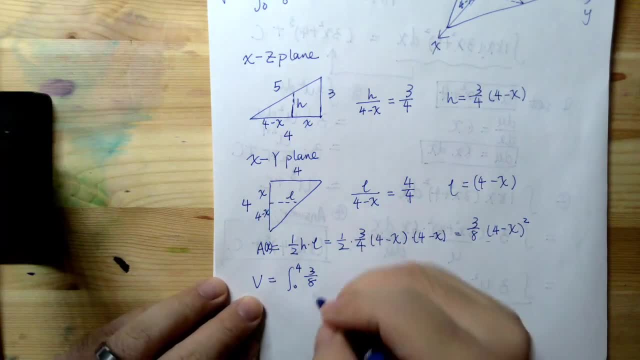 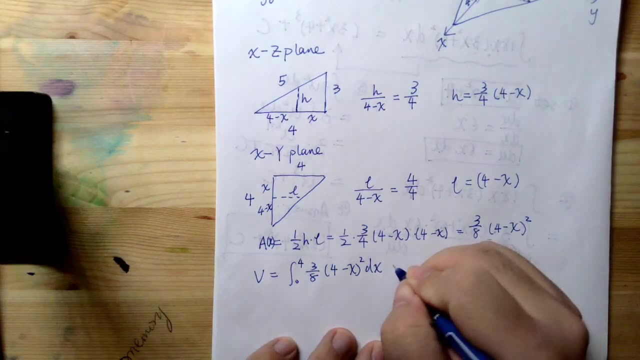 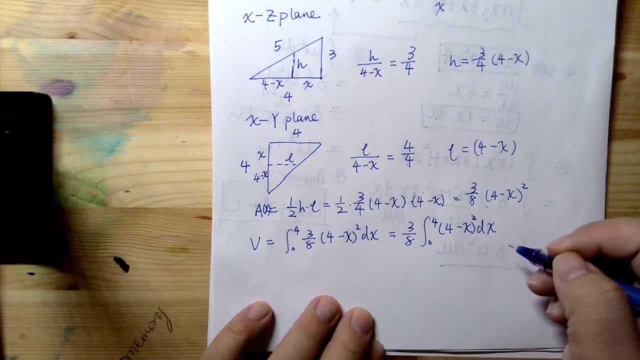 and 3 over 8, okay, and 4 minus X. square DX. okay, we can take this 3 over 8 out 0 to 4. 4 minus X. yes, okay, a lot of square, okay. so we can have two ways to handle this. we can use a simple substitution, or we can expand this and then to 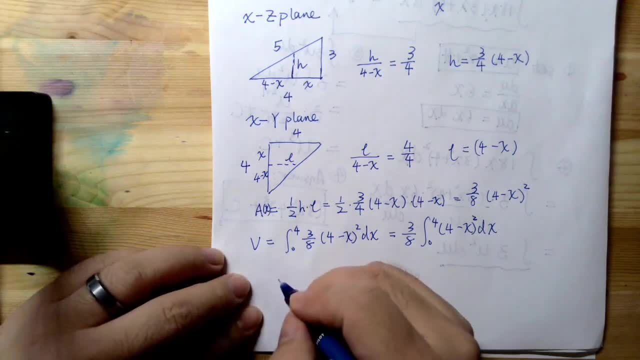 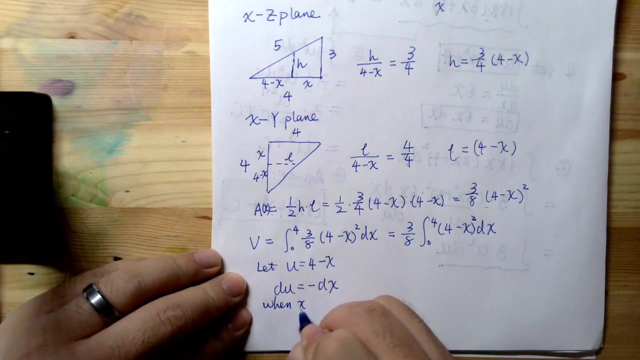 evaluate this integral. maybe we can use a substitution. so let: U equals 4 minus X, okay, then DU equals negative DX. that's something we can tell. and also, when X equals 0, U equals 4. okay, when X equals 4, U equals zero. so with all of this, we can. 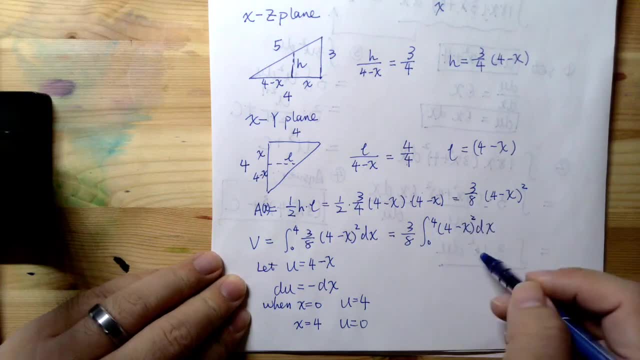 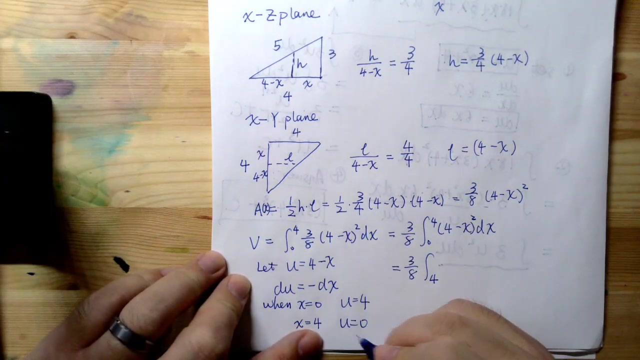 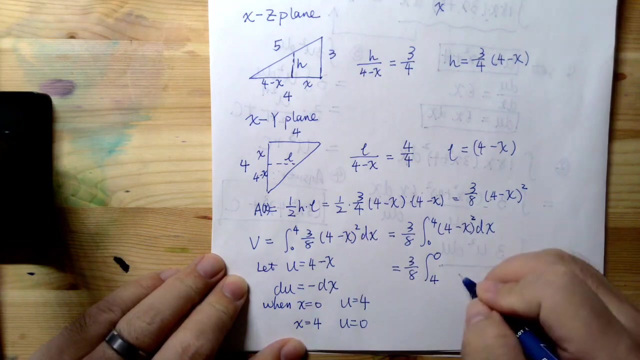 transform our integral into 3 over 8 is still constant and nothing to do with that, and we'll keep that. so remember: yx equals 0, corresponding u is 4. yx is 4, corresponding x equals u is 0. so from 0 to 4, this is, you know. u equals 4 minus x. so here is u, squared, and dx which is going to. 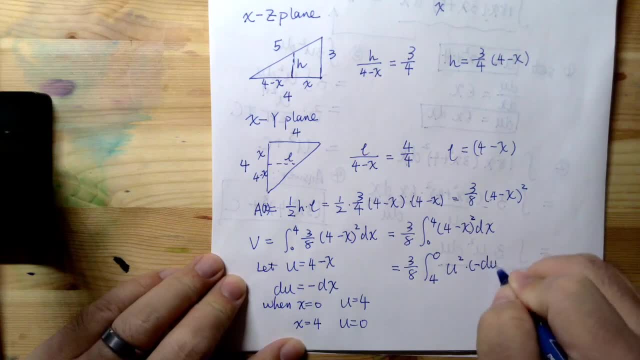 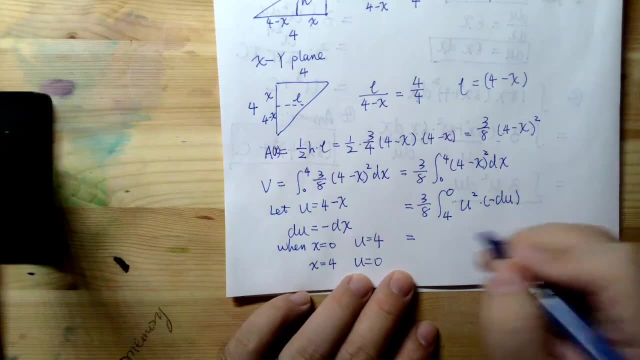 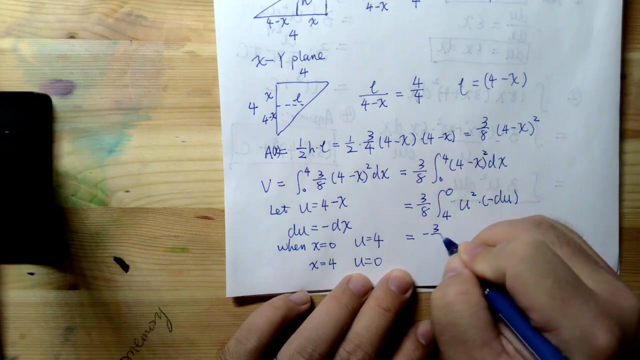 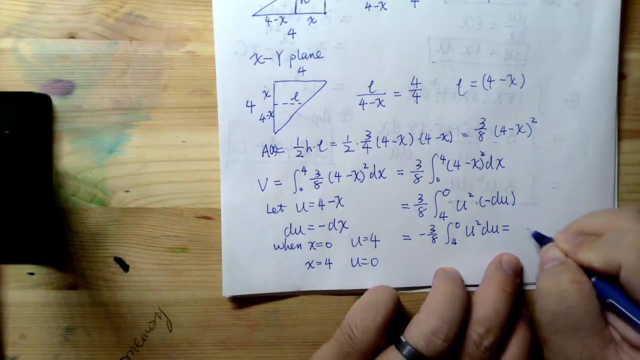 be negative du. okay, so it's negative du. so put all this so we can see we can take this negative in front. this is negative 3 over 8. integral 4 to 0: u squared, du, turns out this is negative 3 over 8. 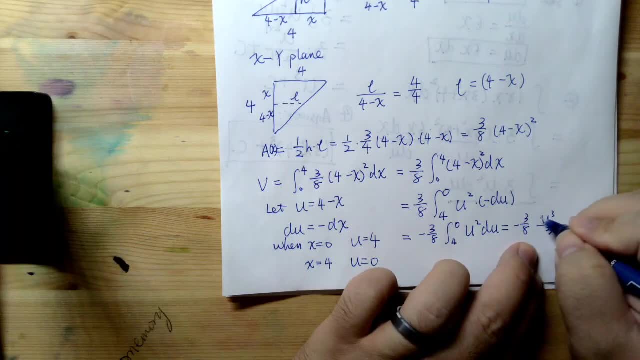 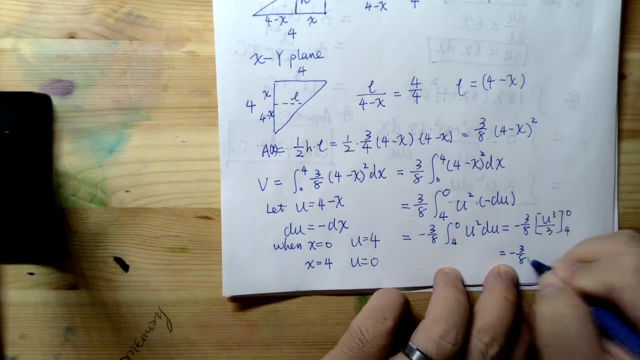 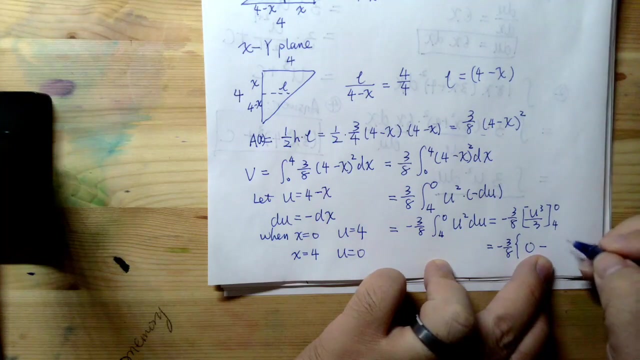 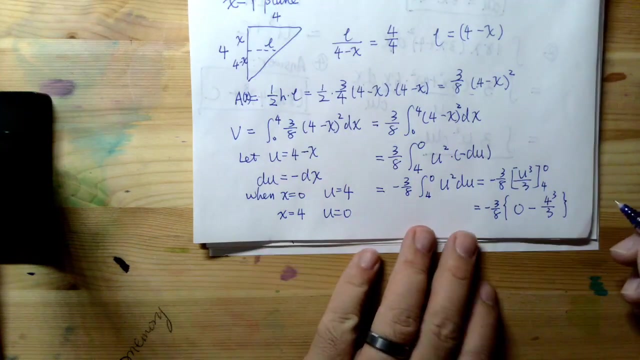 this is u cubed over 3, right, and then. so what we do is block 0, so negative. 3 over 8 is a constant, okay, so okay, so put up 0, so it's 0 minus you put a 4 there, so it's 4 cubed over 3, okay, and then you can simplify this right. 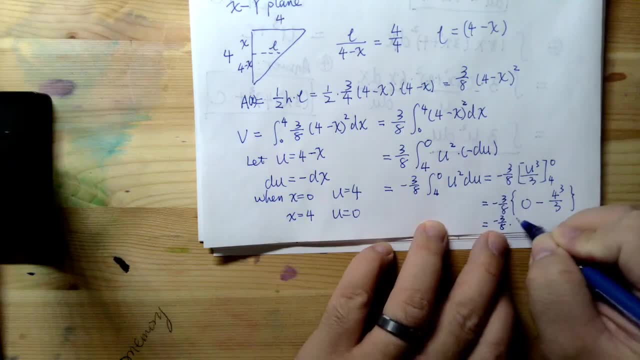 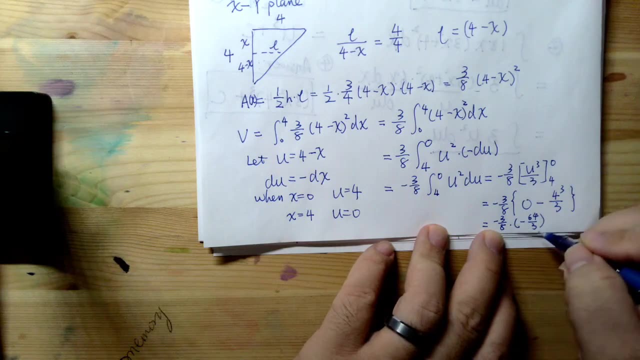 so it's negative. 3 over 8 times negative. 4 over 8, so it's negative. 3 over 8 times negative. 4 over 4. cube is 64 over 3, so it turns out 3 over 3. cancel out negative, negative, positive and then 64 over 8 is 8.